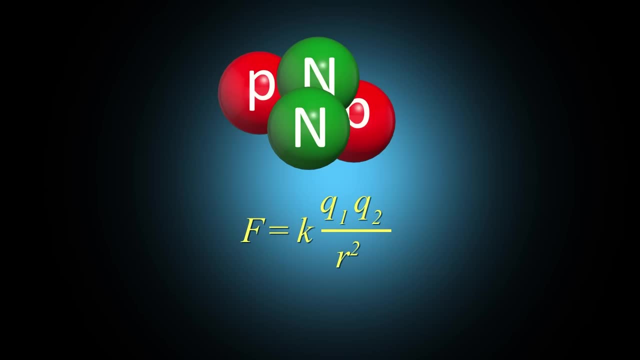 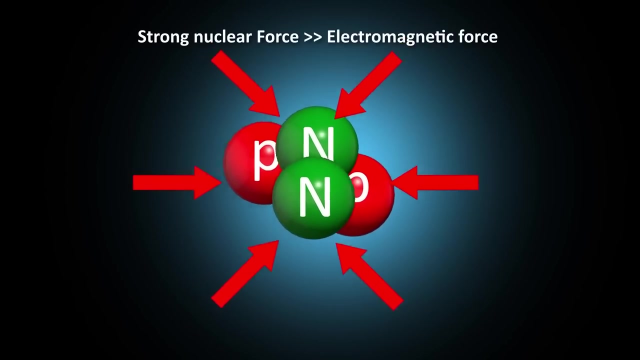 in such close proximity to each other in the nucleus, the electrostatic repulsive force between them is enormous. Two protons, typically separated by the width of a neutron, is on the order of 60 newtons or 12 pounds. But what keeps them together against this tremendous repulsion? 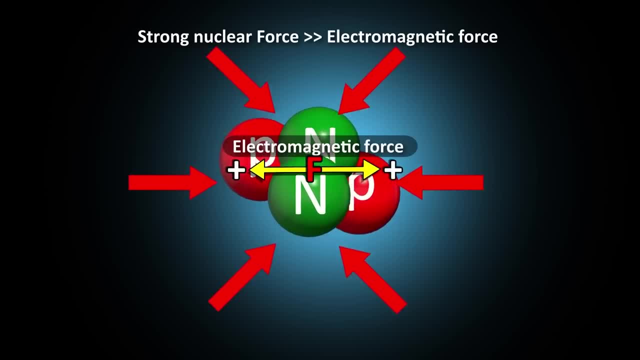 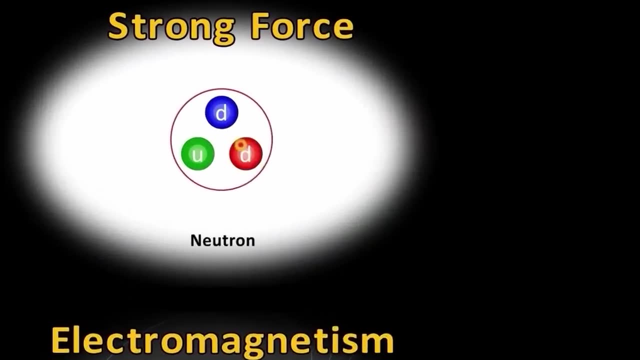 is an even stronger force, called a strong nuclear force, which is about a hundred times stronger than electromagnetism. This force comes from one of the four fundamental forces in the universe- a strong force, But this force, unlike gravity and electromagnetism, operates at very 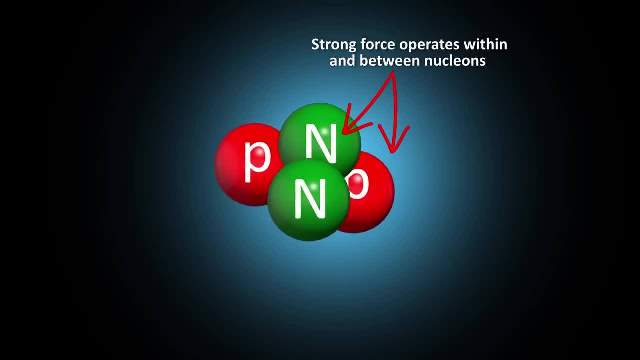 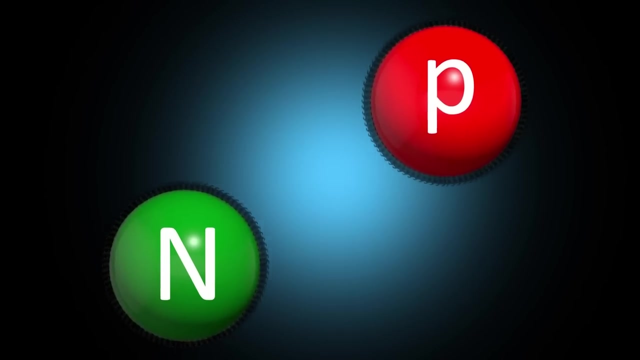 small distances, only about the width of a proton, And it only operates within and between protons and neutrons. Electrons, photons and neutrinos are not affected by it. You can think of the strong force like Velcro, When two objects carrying the strong force are very close. they stick to each other like glue, But if they are far apart, they are unaffected. This means that a nucleus can only grow so large. The reason is that the two opposing forces, electromagnetism and the strong force, operate differently. The strong force only acts at short. 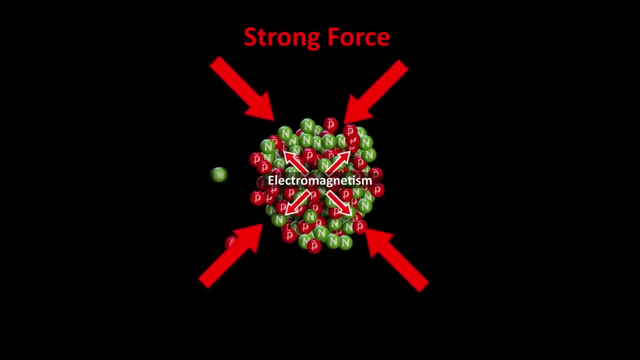 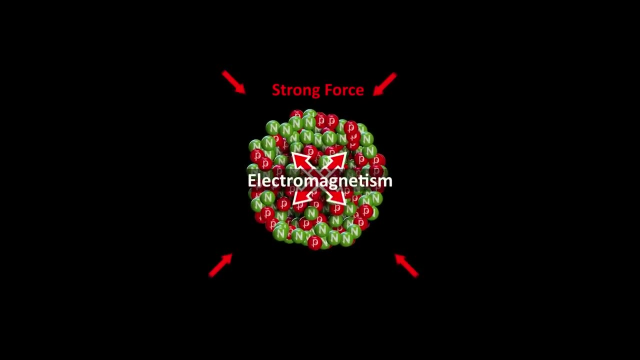 distances. So a given proton or neutron's attractive effect diminishes rapidly as the nucleus grows larger. But since electromagnetism has an infinite range, its force is required to accumulates as more and more protons are added together. So all the protons in a nucleus participate in repelling each other. 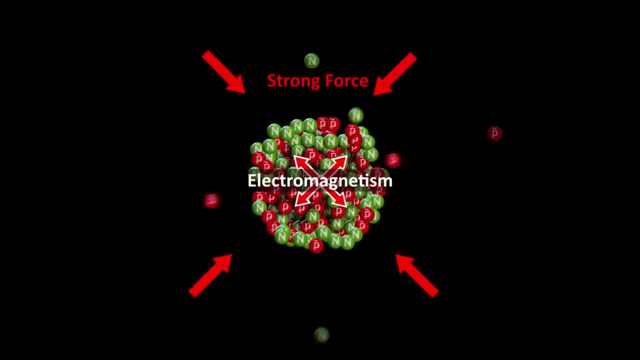 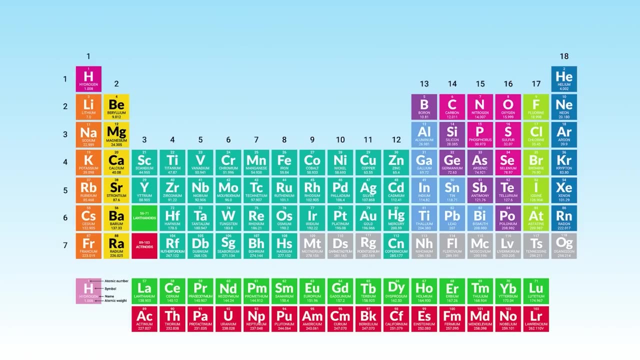 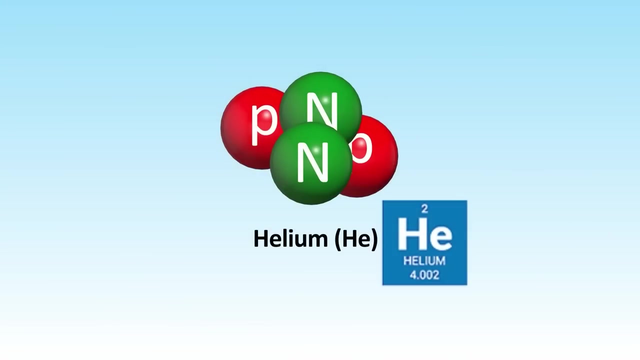 This repulsion quickly overwhelms the attractive effect of the strong force as more protons are added, disrupting the stability of the nucleus. So the heaviest stable element is lead, which has 82 protons. The number of protons in an element is important because it is solely responsible for its atomic 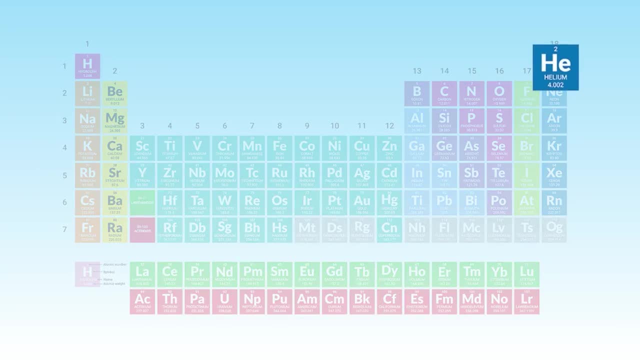 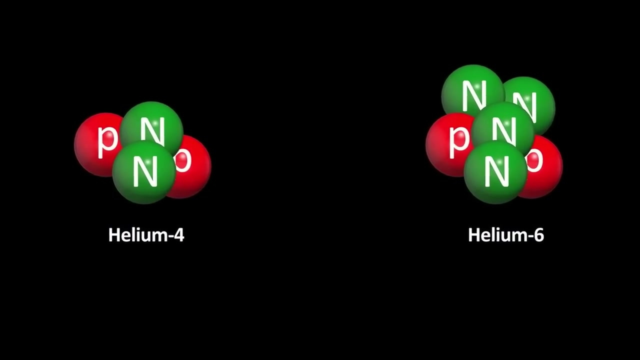 properties. The proton number corresponds to the position of the element on the periodic table. A given element or atom can have the same number of protons but different numbers of neutrons. These are called isotopes of the element. They have exactly the same physical and chemical properties but differ in mass. 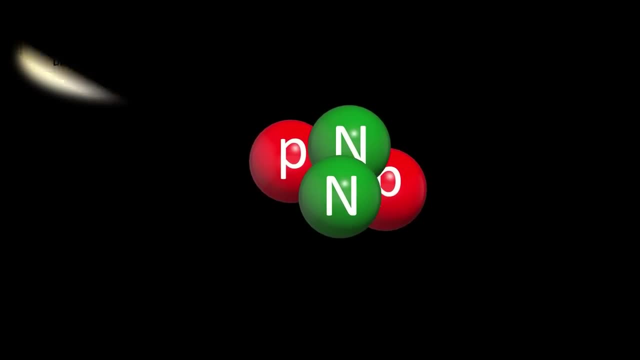 Stable nuclei consist of roughly the same number of protons and neutrons. The neutrons serve to provide a additional strong force needed to keep the nucleus stable. Without neutrons, not even two protons can be held together against their repulsion. Free protons are stable, but free neutrons are not stable. 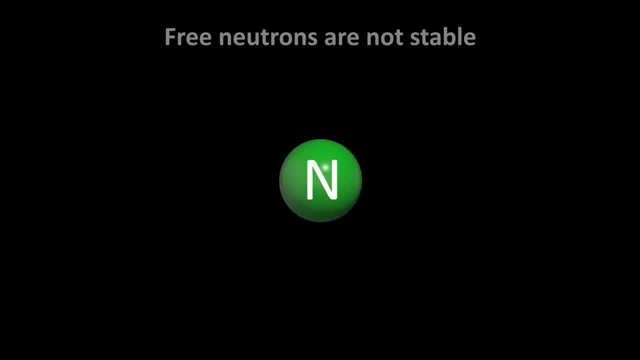 Low neutrons decay into a proton, an electron and an antineutrino within about 15 minutes, But inside the nucleus they remain stable because it is energetically unfavorable for them to decay. In other words, the energy gained from a neutron's decay is less than the energy gained from 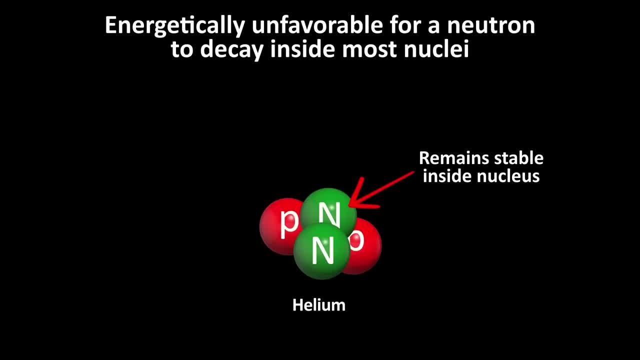 a neutron's decay. A neutron decaying to a proton is lower than the increased energy required to keep an additional proton in the nucleus if there are plenty of other protons around. But this type of neutron decay in the nucleus is not impossible and can happen in very neutron-rich. 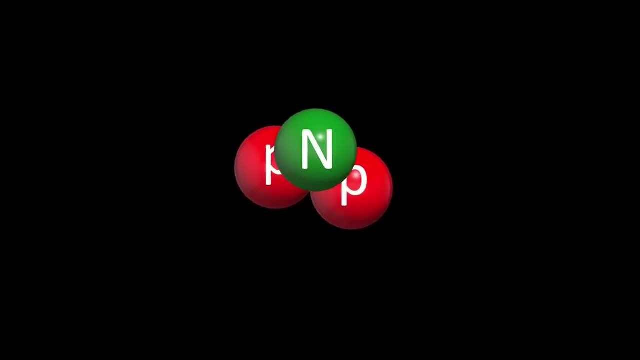 isotopes of a given element. But a nucleus cannot have too few neutrons or the nucleus will not be stable. It also cannot have too many neutrons because eventually the strong force can no longer keep them from decaying into the nucleus. 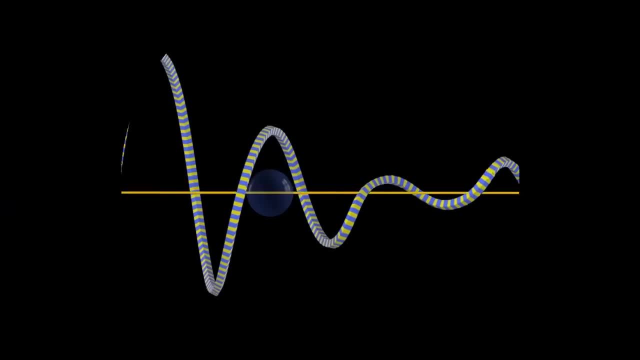 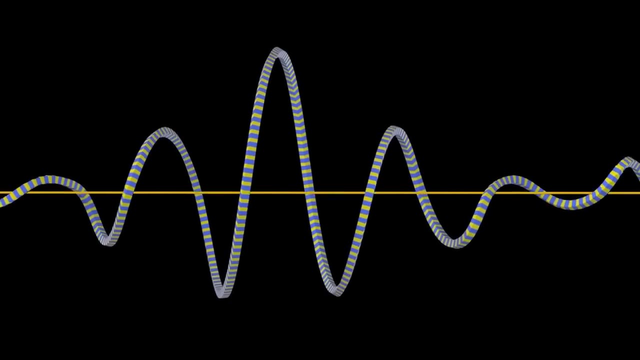 It will just keep decaying into a proton and forming a different element. Protons and neutrons, just like all quantum objects, are subject to the laws of quantum mechanics. One consequence of this is that quantum particles have a very small but non-zero probability. 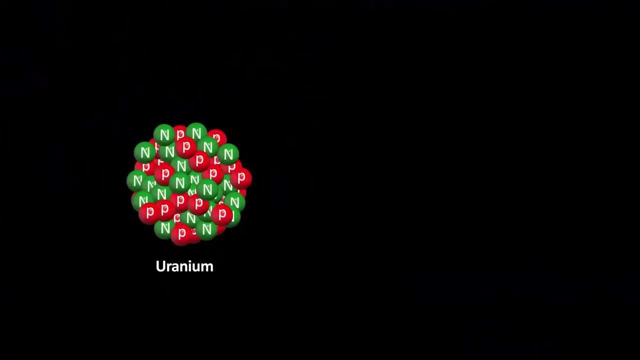 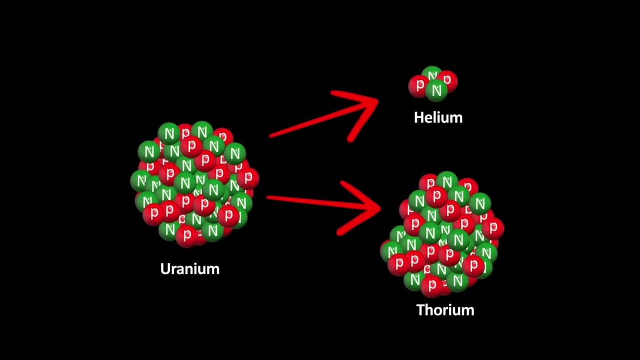 of appearing anywhere in the universe. The reason I mention this is because it is tied to a certain kind of natural radioactivity called alpha decay. If a nucleus is very large or has an excess number of protons and neutrons, it is likely. 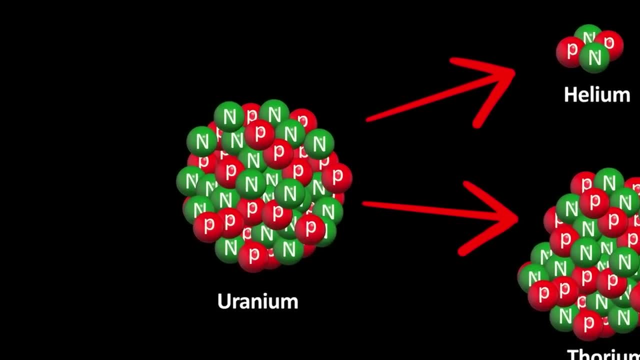 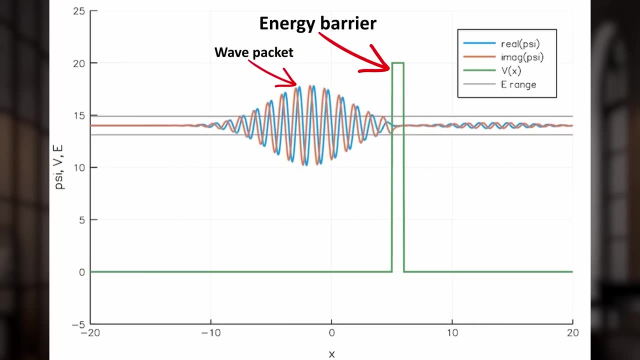 to decay. If a nucleus is very large or has an excess number of protons and neutrons, it is likely to decay, And the strong force can barely hold it together. Quantum objects have a higher probability of appearing on the other side of an energy. 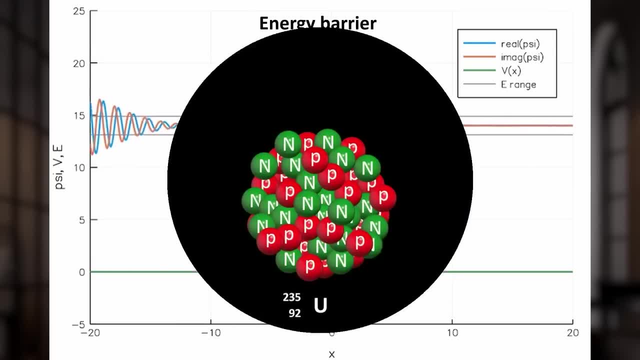 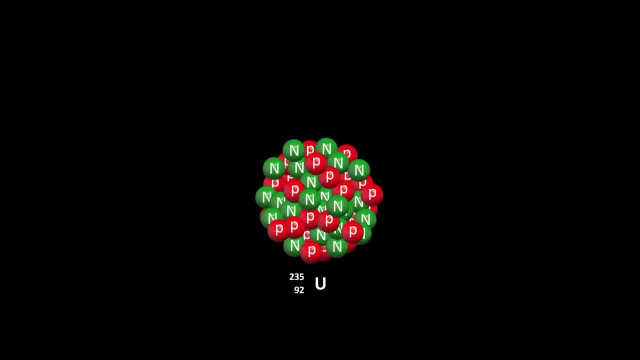 barrier. if the barrier is not very high In the case of very large nuclei such as uranium, the energy needed to liberate protons and neutrons is small enough that, sooner or later, an alpha particle, which is essentially a helium nucleus consisting of two protons and two neutrons, can quantum mechanically. 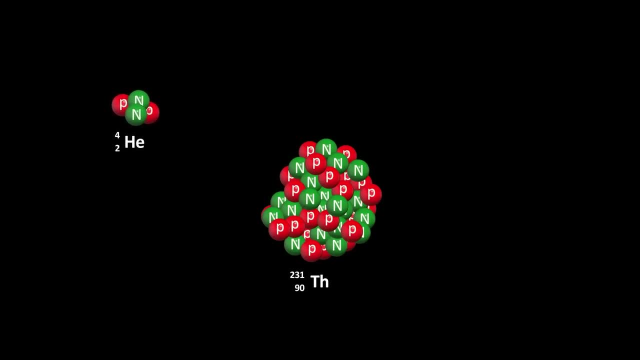 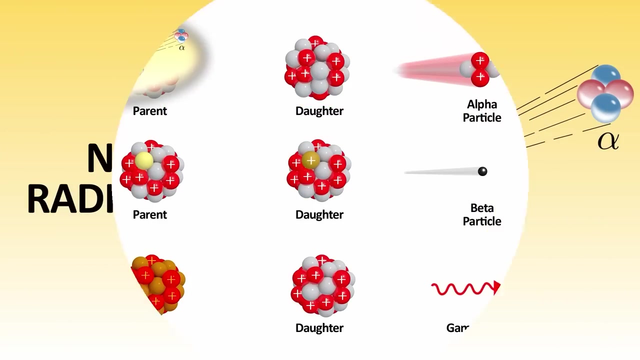 tunnel through the strong force barrier And appear outside the nucleus, Then they speed away very fast. This is what we call radioactivity. If you want to learn more about quantum tunneling, I have a video on that right up here. There are three forms of natural radioactivity: alpha, beta and gamma decay. 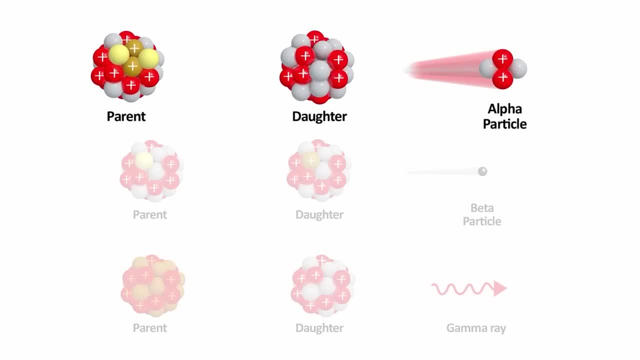 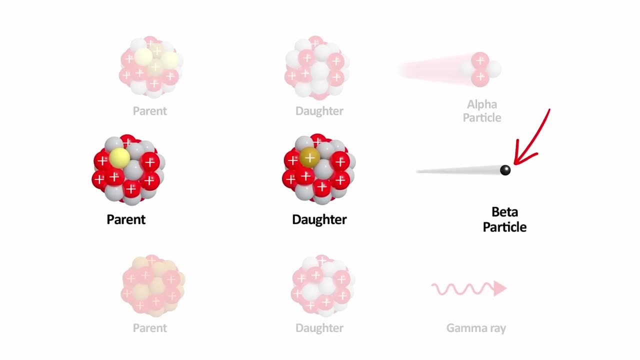 An alpha particle consists of two protons and two neutrons. This type of radiation happens via the mechanism I just described. The beta particle is a high energy electron In some very large nuclei that might be barely bound together. a second fundamental force, called the weak force, can compete with the strong force and cause a neutron to decay. 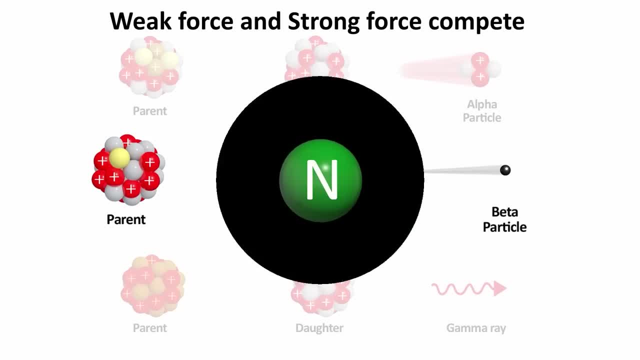 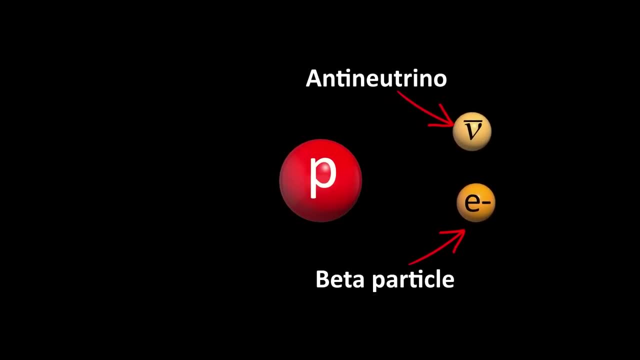 even though it is in the presence of protons. As I said before, when a neutron decays to a proton, it gives off an electron and an antineutrino. This electron that it gives off is the beta particle. A gamma particle is a high energy photon. 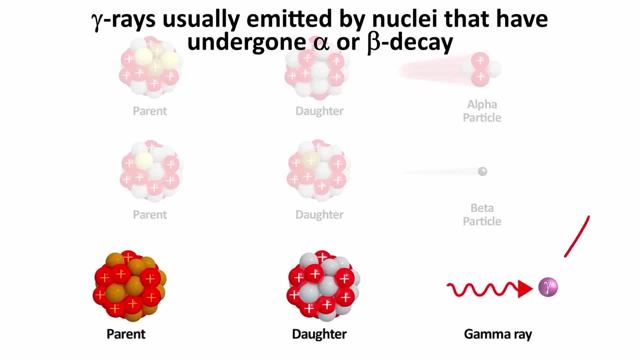 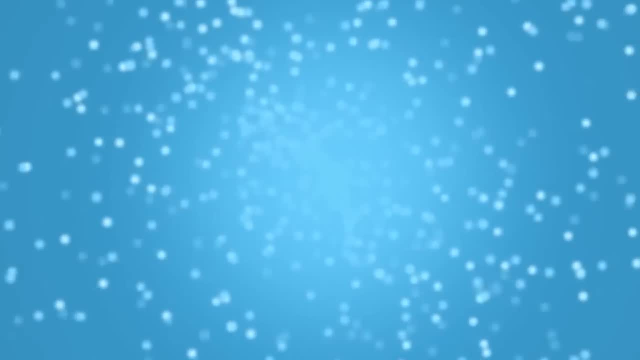 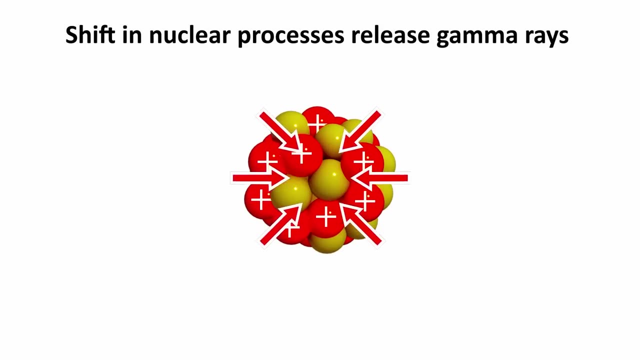 Also called a gamma ray. Gamma rays are usually emitted by excited nuclei that have been created after either an alpha or beta decay. The reason these processes release such high energy photons is because they involve nuclear processes, which are due to the strong force, And since the strong force is so much stronger than, for example, the next strongest force, 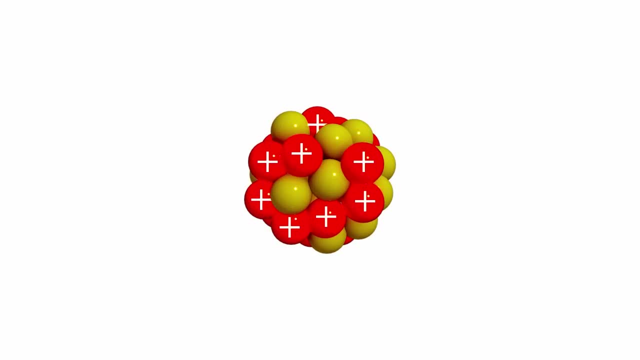 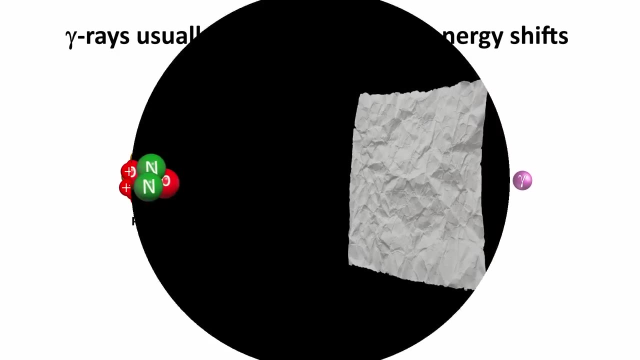 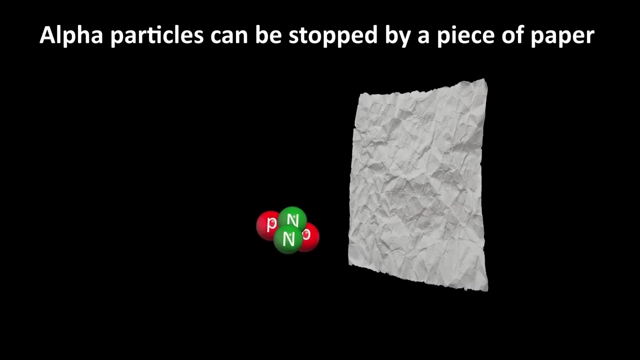 electromagnetism. whenever there is a shift to lower energy levels within the nucleus, an enormous amount of energy is released, and this high energy is in the form of gamma rays. The three forms of radioactivity have very different abilities to penetrate matter. Alpha particles can be stopped by a thin piece of paper. 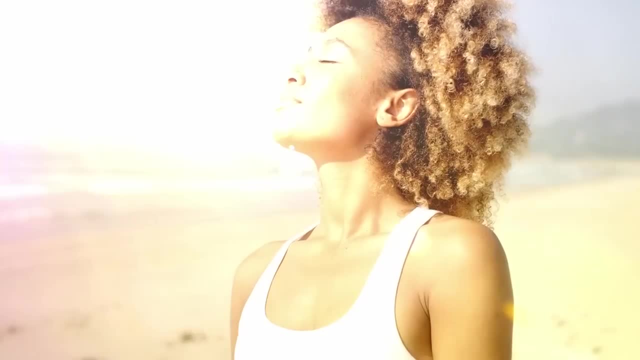 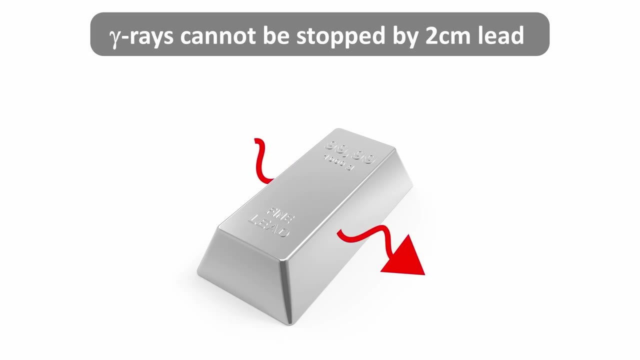 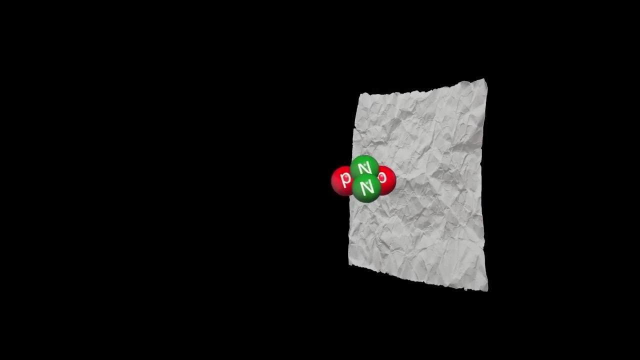 Beta particles can penetrate your skin but can be stopped by a thin sheet of metal like aluminum foil. But gamma rays are very difficult to stop and can penetrate through even an inch of lead. Why is this the case? Alpha particles, consisting of two protons and two neutrons, are relatively big, heavy. and thus slow. Because of their large size, they can be easily blocked. Beta particles travel much faster and can penetrate matter more easily because of their higher velocity and smaller size. Gamma rays have no charge and they are moving at the speed of light. These photons pretty much have to hit a nucleus directly to be stopped. 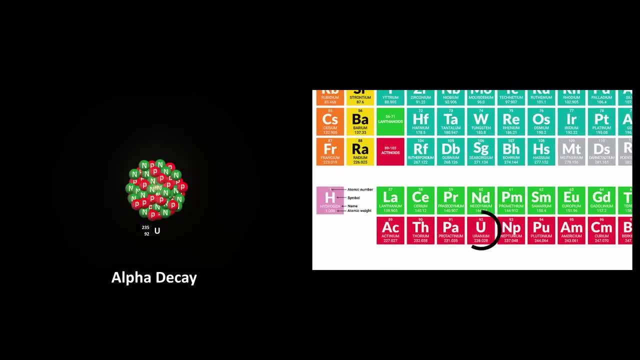 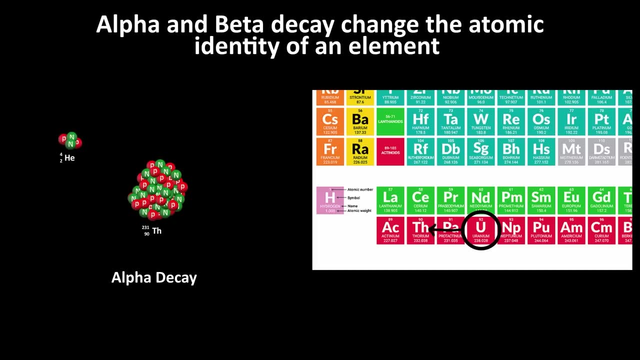 Alpha and beta decay change the atomic identity of the decaying nucleus because they change the number of protons. Alpha decay subtracts two protons, so the element moves down two notches on the periodic table. Beta decay changes a neutron into a proton or vice versa, so it changes the type of element. 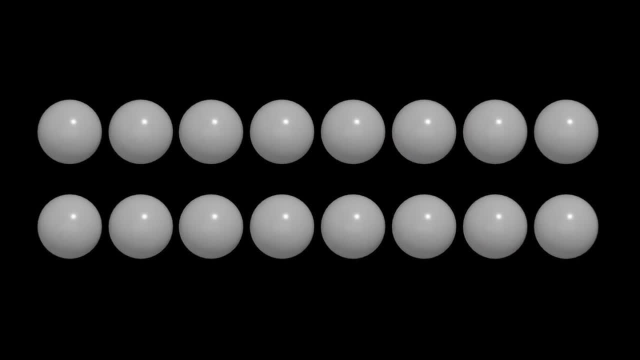 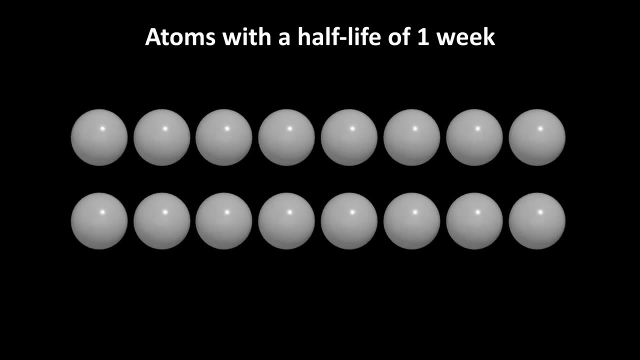 either up or down. A radioactive nucleus is characterized by something called its half-life. What this means is that if I have a certain number of radioactive atoms, let's say 16 atoms, and its half-life is one week, then one week later I'll have half of this, or 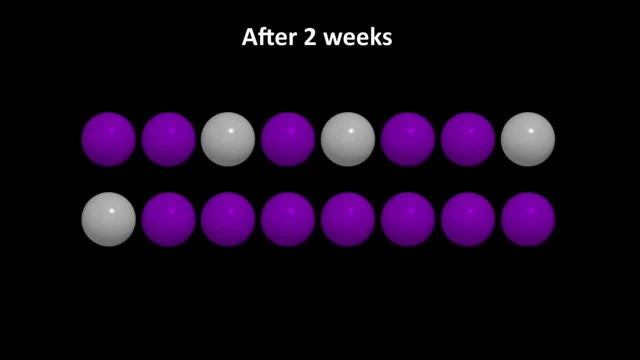 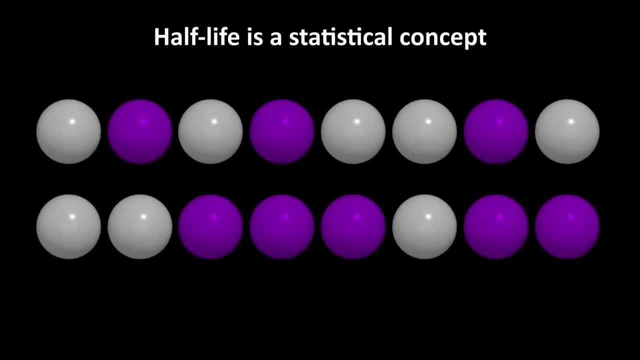 8 atoms remaining, And in two weeks I'll have half of that or four of the original atoms left, And this goes on. Half-life is a statistical concept. If you are holding the 16 atoms, you will not be able to determine which of the atoms will. 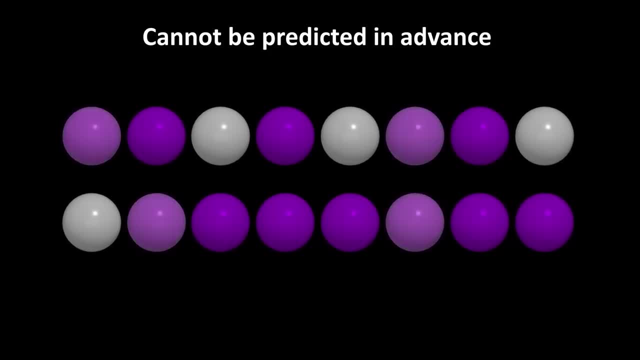 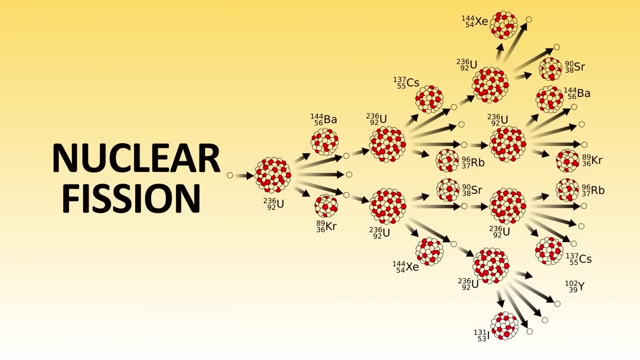 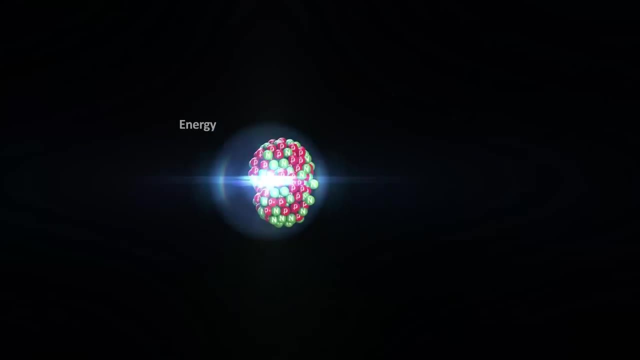 decay one week from now or a billion weeks from now. You can only say that any given atom has a 50-50 chance of doing so in the time of one week. If a Large Nucleus, like some isotopes of uranium, like U-235, is hit by a particle, usually a neutron, then it will be split into. 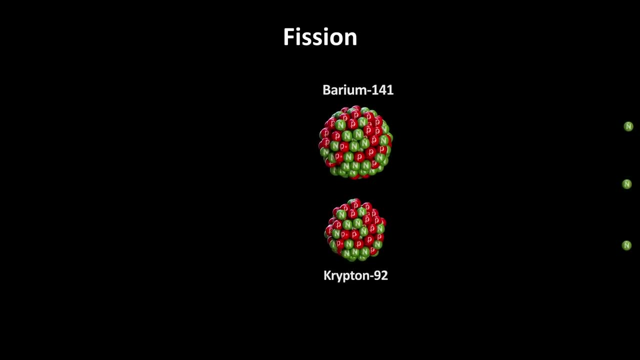 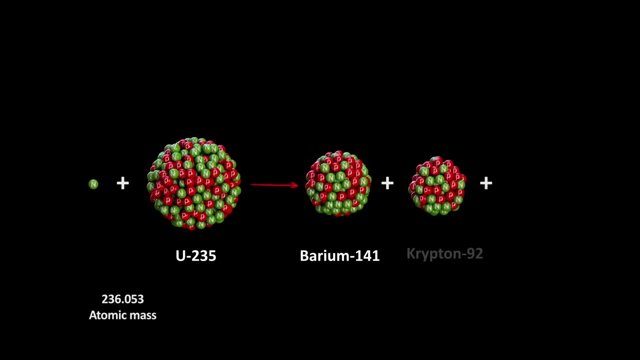 two smaller nuclei. This is called nuclear fission. If the total mass of the two smaller nuclei is less than that of the uranium before it was hit, the missing mass is turned into energy via the equation E equals mc squared In the case of certain isotopes of uranium and plutonium, such as U-235 and plutonium-239,. 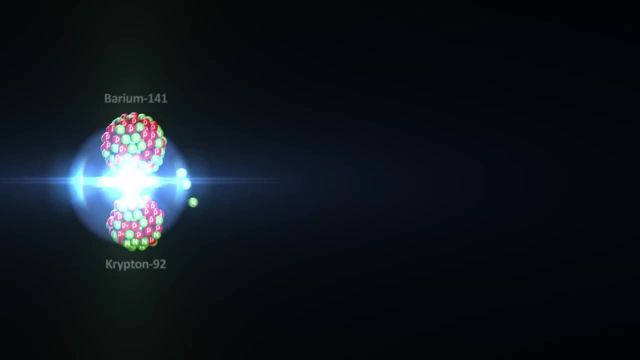 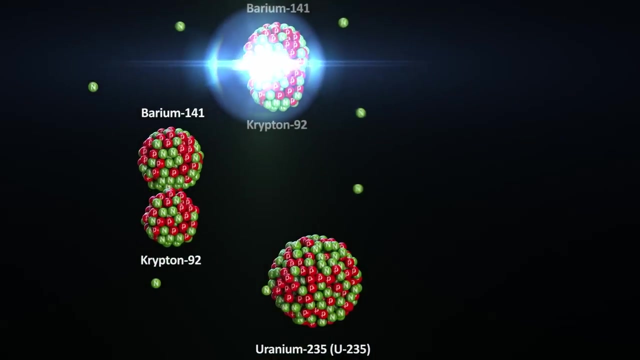 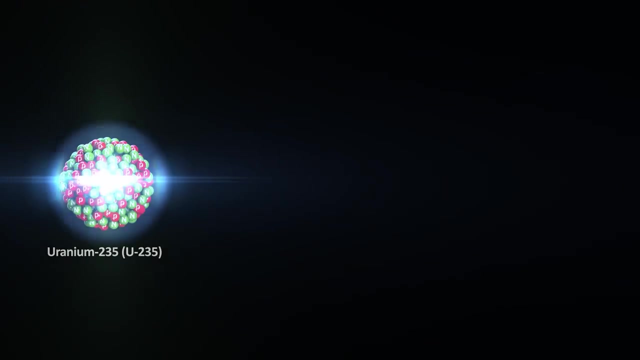 when these are hit by a neutron, they split into two lower mass nuclei and three neutrons are also thrown off. If there is enough fissionable nuclei in high enough concentrations, then it is possible for the three thrown off neutrons to in turn fission three more nuclei. 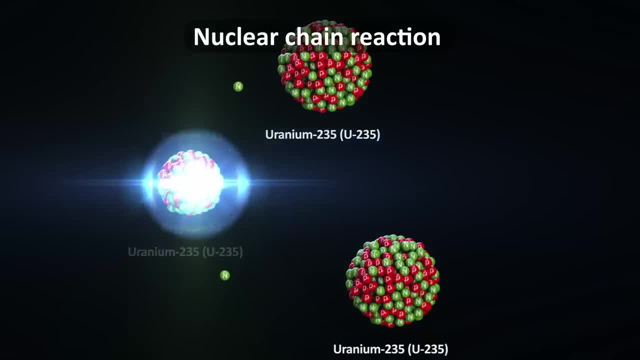 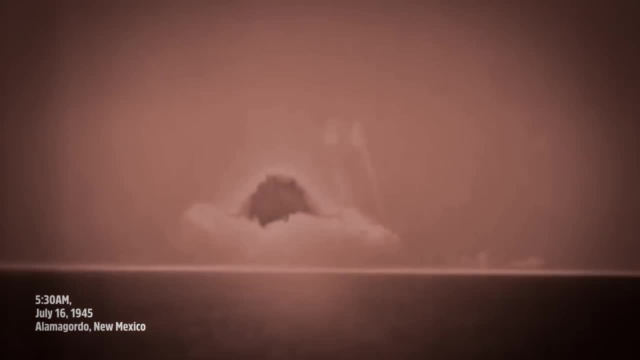 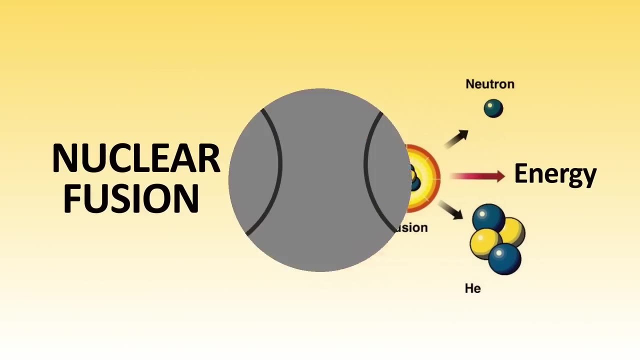 Which, in turn, fission nine more nuclei, Which, in turn, fission 27 more nuclei, Creating what is called a chain reaction. This is the mechanism behind the atomic bombs dropped on Hiroshima and Nagasaki- Hiroshima and Nagasaki during World War II. 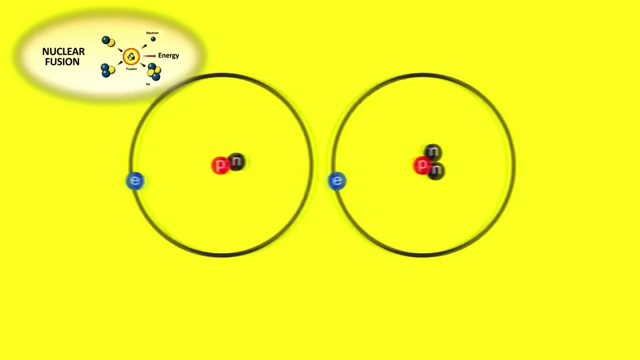 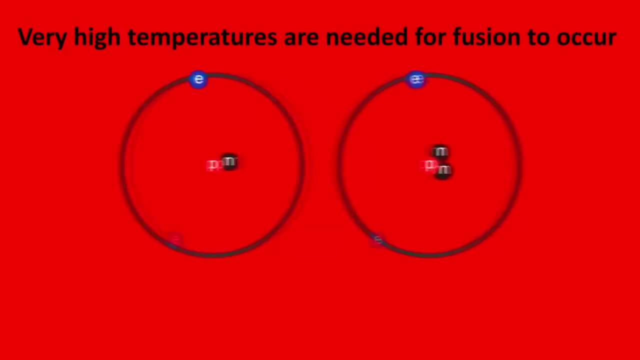 A kind of opposite of fission is fusion. This happens when two small nuclei, such as hydrogen, which consists of only a single proton, can be brought close enough together that they fuse into a single nucleus. Fusion is very difficult to achieve because the protons strongly repel each other. 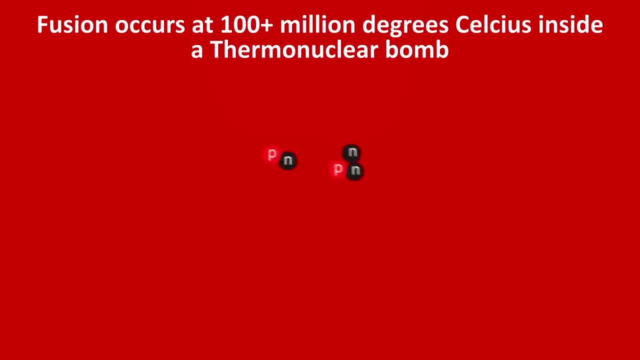 Only gases heated to millions of degrees Celsius have atoms moving fast enough so that they can approach each other close enough to achieve fusion. Quantum tunneling also plays a role here. A hydrogen bomb achieves very high levels of energy release by using the heat of a fission.